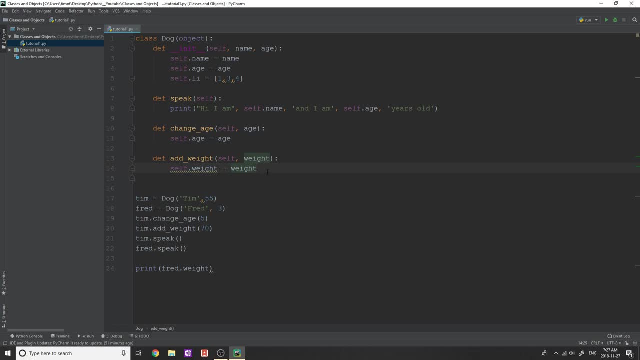 objects. I just want to start off by quickly saying, though, if you guys are finding the video is a bit too slow for you- and I'm kind of explaining things a lot of time- the reason I do that is because I'm not sure the level of person that's going to be watching the video, and I want 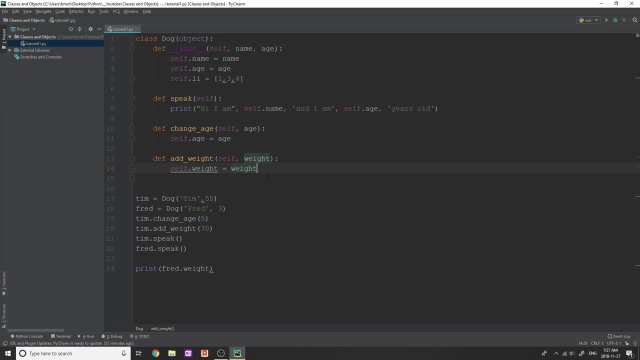 to make sure that the people that will understand quickly can get the information within like the first few minutes, And then the people that really need some extra reinforcement have that opportunity to watch through the entire- like 11 or 12 minutes- and have it explained to them. 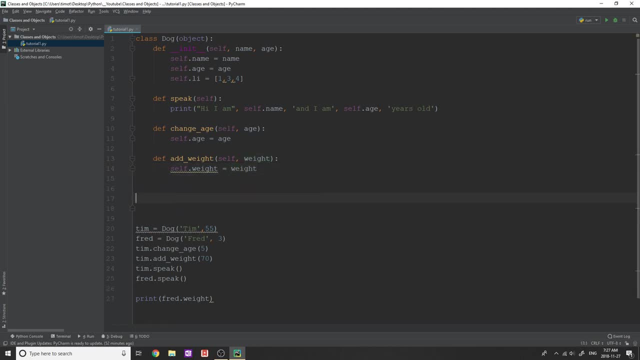 multiple times. So if you guys are finding it's a bit too slow and you want to move faster, just fast forward the video or skip to the next one. if you guys are done with whatever I've been talking about, Because, like in the last video, for example, I watched it back And I kind of 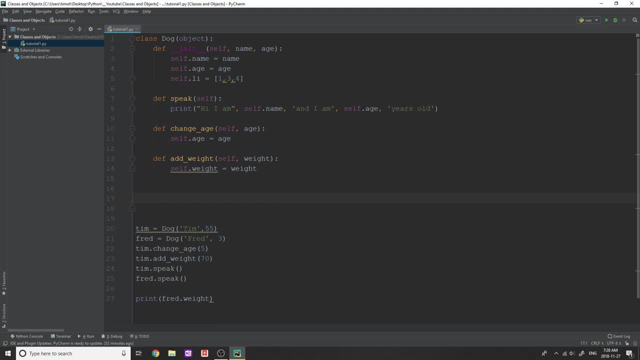 explained the same thing a few times. That's just for the people that need a bit of information. So if you guys are finding it's a bit too slow and you want to move faster, extra help And that's kind of what I aim to do with a lot of my videos, so that people that need 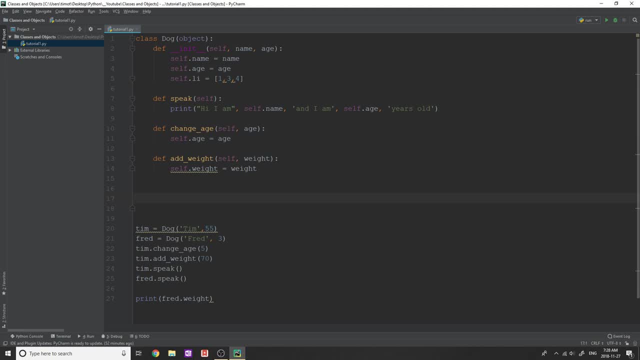 help. can you know, grab that if they want to. okay, So let's get started And I'm just going to modify this dog class. just delete li, we'll get rid of change age and add weight And we're just going to have name, age, so on, like that, okay, and we can get rid of all this stuff down. 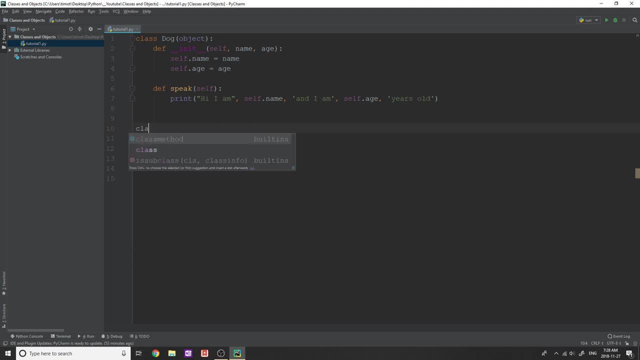 here. Now what I'm actually going to do is I'm going to create a new class And I'm going to call this cat. Okay, now, cat is going to have very similar attributes as dog, In fact. let's just copy them over. Okay, so we'll paste them like here: we have name. 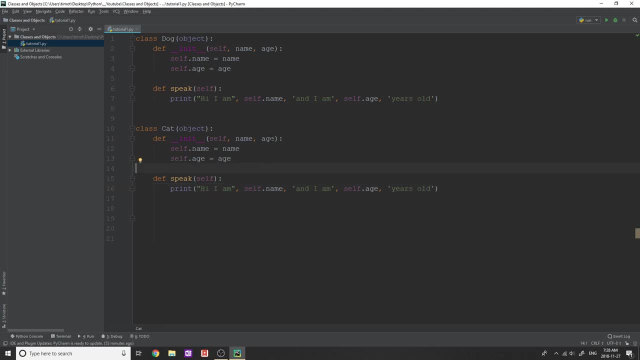 age, hi, I am whatever. Okay, now I'm just going to add one thing, And in this case I'm going to add: let's see color. okay, today self dot color is equal to color. Okay now, this cat object is: 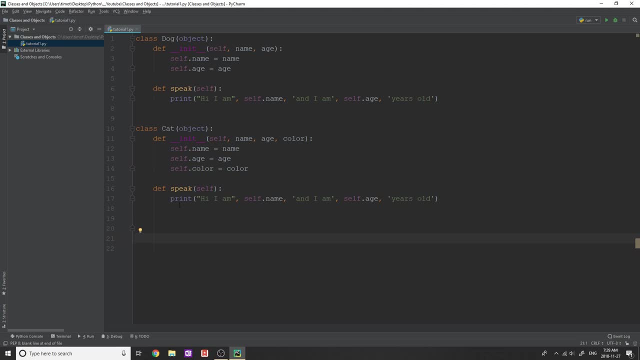 obviously going to work the same as dog. I don't think I need to show you Now. just take note of what I just did. I just copied all of the stuff from here into cat. Now if you know anything about programming, you know that programmers don't like to copy and paste and that you really 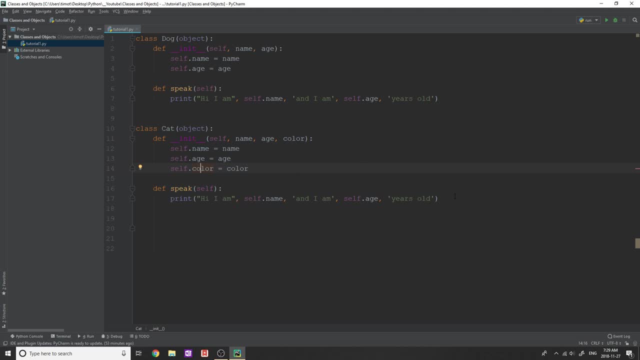 shouldn't be copying and pasting code. So Python has actually come up with a solution to what I just did that allows us to not have to do that, And that is called inheritance. So I'm going to delete all this And I'm going to go back into cat And I'm going to type dog here. Now what? 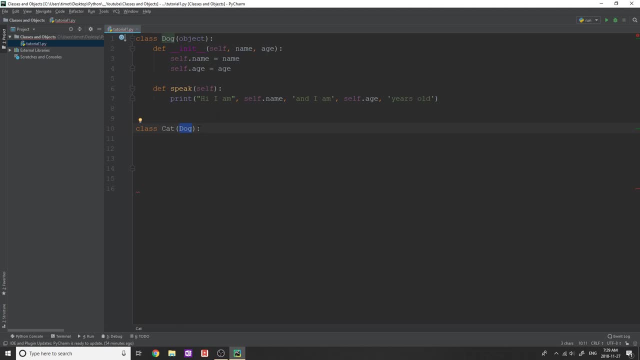 this little bracket up here means is. it means parent. So whenever you're talking about inheritance, you always have a parent or a superclass And then you have a child or a like derived class. So you're going to have a parent or a superclass And then you have a child or a like. 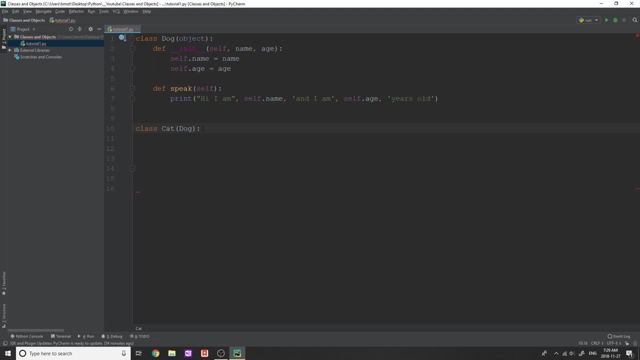 class. Okay, and there's a bunch of different words for them. They're not really that important, Just no parent and child. It's the most basic, Okay. So in this case cat is going to inherit from dog, which means dog is the parent class And cat is the child class and it is derived. So 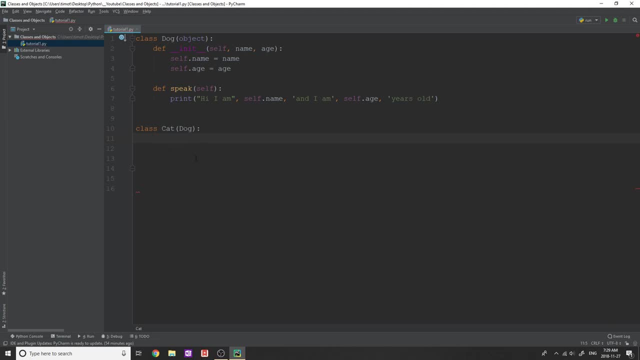 it's taken from dog. So that means if I do class dog and if all I do in here is just type one thing, so I type net, underscore, underscore, And in here I'm just going to put name, age and color And I'm just going to do that, And I'm just going to put name, age and color And I'm. 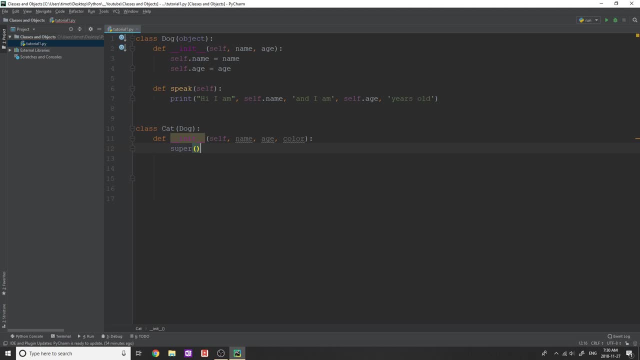 just going to do something that's going to look confusing. I'm gonna explain it. after: Okay, super dots, underscore, underscore, underscore, underscore, underscore, and I give it name, age, say, self dot color equals color, And then I create a new object of cat. So I'm just gonna say: 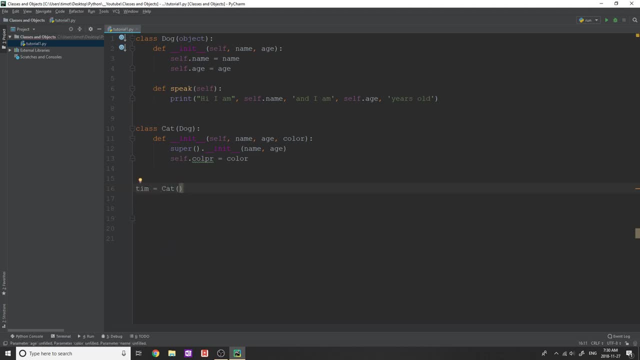 Tim equals cat. give it a name: agent colors. In this case we'll do Tim, age five. color: blue: blue cat. I know okay, So we do that. We press play, no errors. Okay, I'm just gonna show you if I do Tim dot speak. 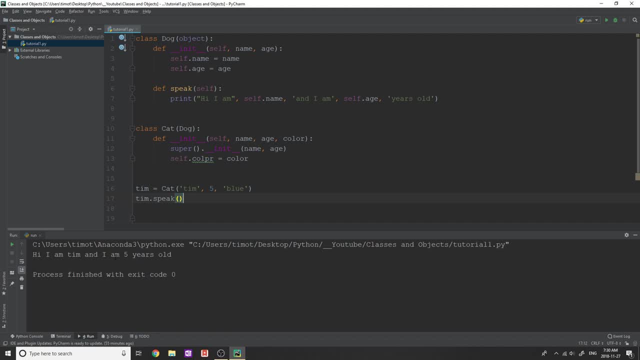 what do you think is going to happen? Take a guess. It says: Hi, I'm Tim and I'm five years old. Now, how the heck does all this work And what did you just do? I know that's probably. 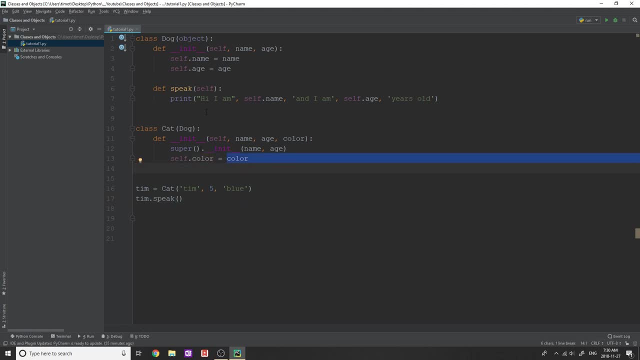 the question you're asking Probably fix that, say color. So the way this works is when you inherit from another object or another class- sorry- you actually inherit all of the properties and attributes and methods of that class. So when I do that, I'm going to say hey, I'm going to do. 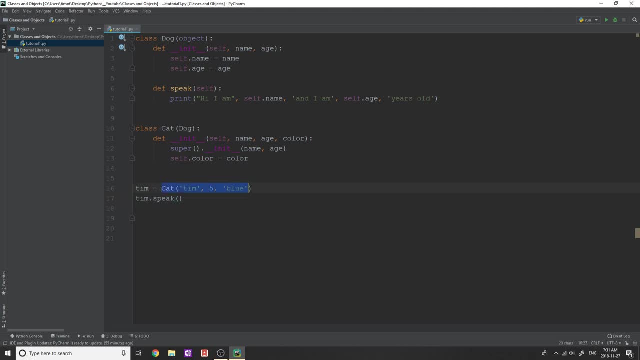 Tim dot speak. you can see, well, Tim is an object of type cat and cat. Well, I don't see speak here. How does that work? Well, since the speak method belongs already in the dog class and we're inheriting from the dog class, it is actually carried on to the cat class and we're able to. 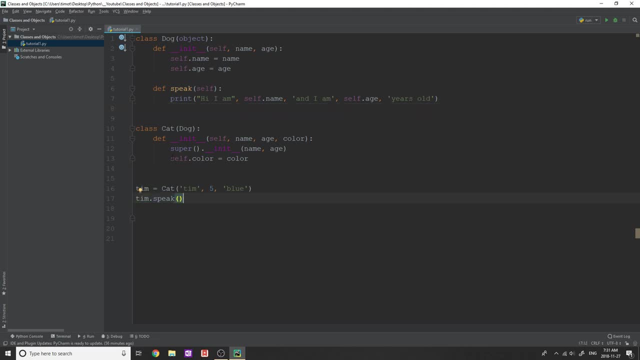 use it like that. Okay, so Tim dot speak. Now what I did here with this super dot init. I know this looks confusing, but pretty much in the initialization of cat, which is, you know, you're unique to cat because it has this added parameter color, I simply called the initialization of dog. 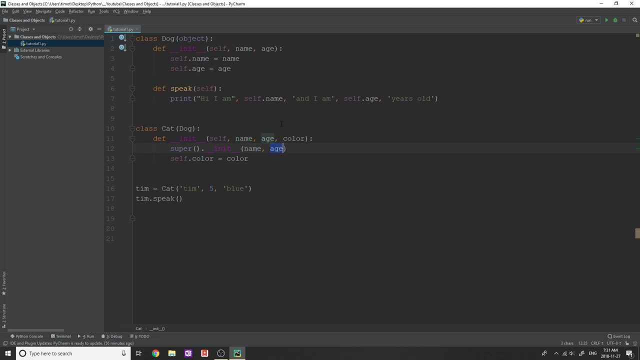 first, which means that when I gave it name and I gave it age, it automatically added self dot name and self dot age to my cat object of Tim. You see how here I didn't type self dot name equals name. I didn't type self dot age equals age. All I did was call the constructor method or the 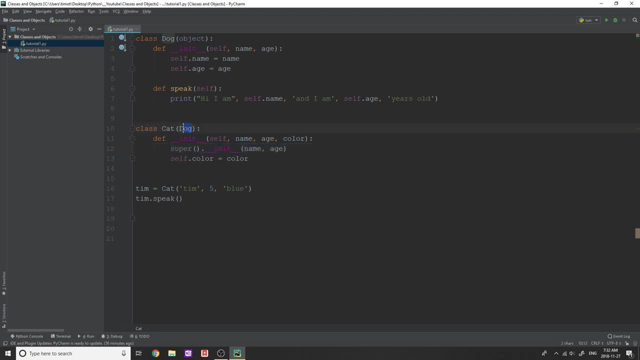 initialization method of the super class, and the super class simply means dog, And it did that for me. Now, in this example, it seems like: well, why in the world would you want to do that? That like that doesn't make sense. There's not that many lines, whatever. If you. 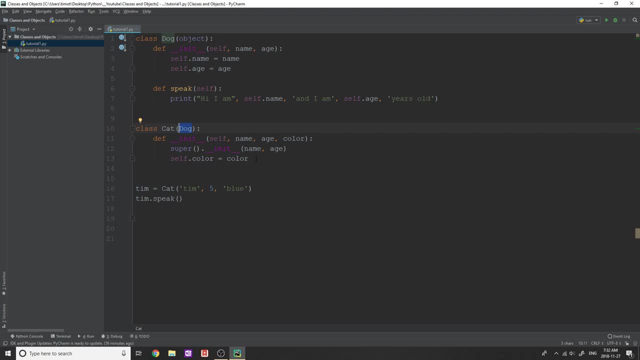 have really long methods and really long classes, it makes a lot of sense to inherit. So in this example it's hard to show, but in long ones you do want to inherit. Now I want to show you that you can add and overload things from the parent class. So, for example, the parent class has speak. 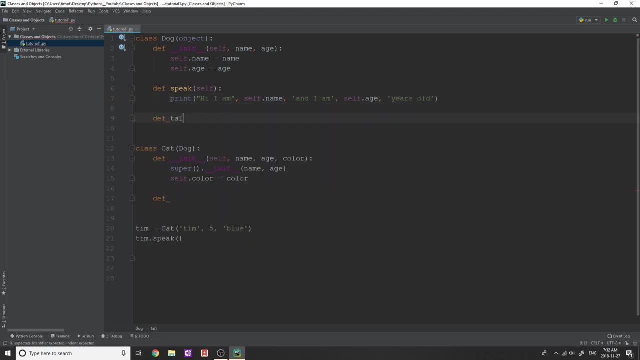 I'm going to add one more method in here. say define, let's just say talk, okay. And here it's going to say print: bark because it's a dog, Okay. Now, obviously in our cat class, if we want to talk, we don't want to bark, right? And 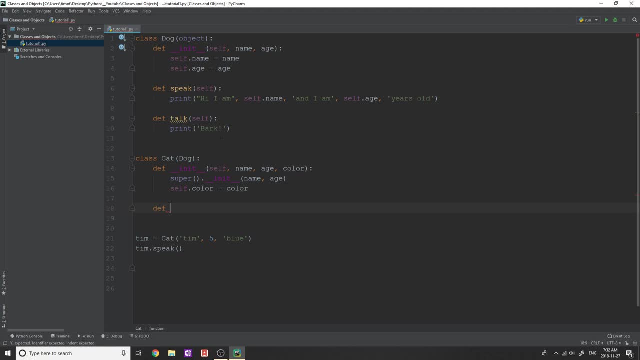 that's what's gonna happen right now. If we do Tim dot talk, it's just gonna say bark. So if we wanted to change this, we can actually overload this, override this method. So if I do define talk in here I can print And in here and I'm not going to. 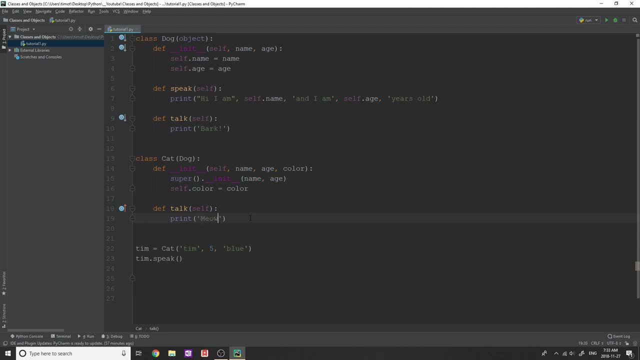 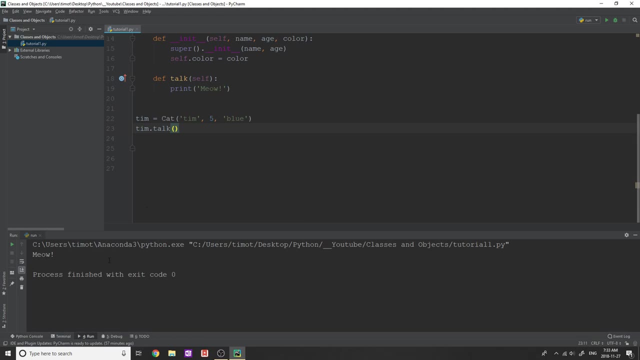 do bark, I'm going to do meow. Okay, like that little explanation point. So now, if I do Tim dot talk this, you can see that we get meow instead of bark, And that goes for anything in inherited classes. Okay, So anything that we do in here is going to override whatever is happening in this. 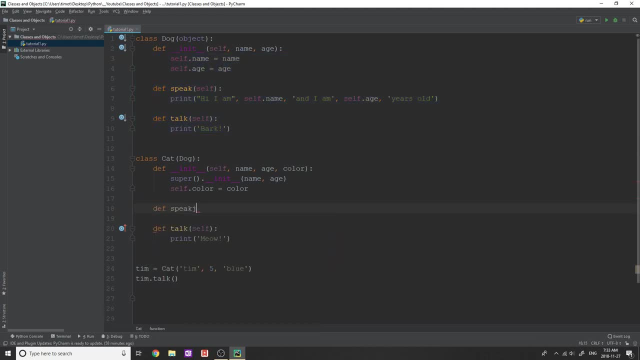 dog class. So say we wanted to change speak. we could say: define speaking here, And then whatever we put in this speak method would overwrite what's in here. Now, that's not to say that it's going to change if you create a dog dog object. So 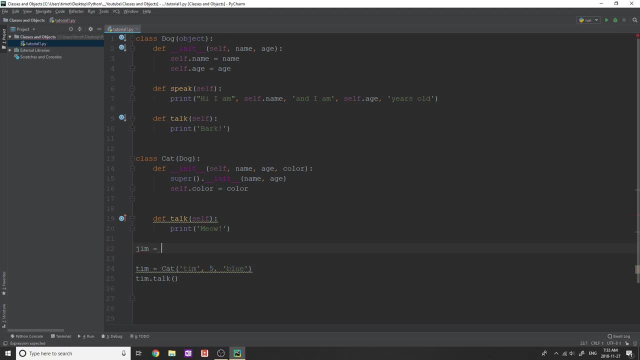 if I do like I don't know. let's say: Jim is equal to dog. give it a name. give it Jim clearly age: it's an old dog, 70. Okay, And we do Jim dot talk. Well, we're still going to get if I spell Jim. 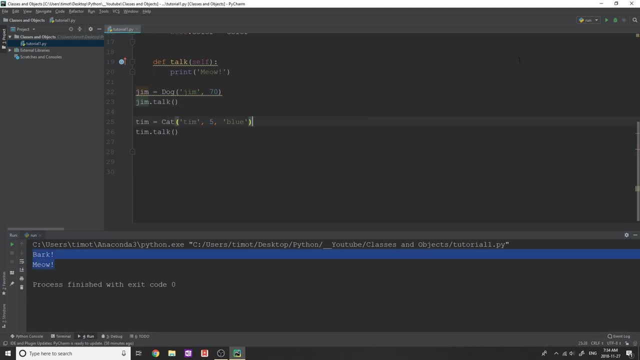 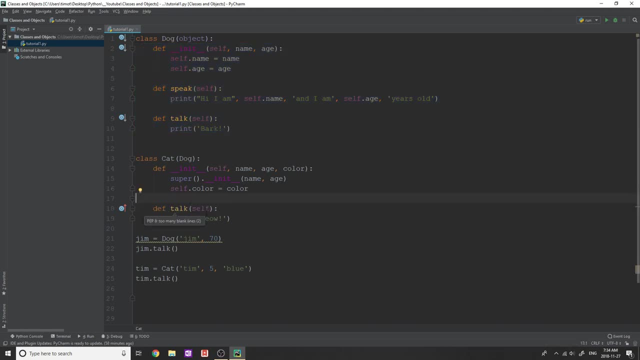 correctly, bark, right, So we get bark, And yeah, so we don't actually change anything In this class. we just say that, well, if you create a class on, or if you create I can't object, then it's going to have this talk method which overrides the talk method that we 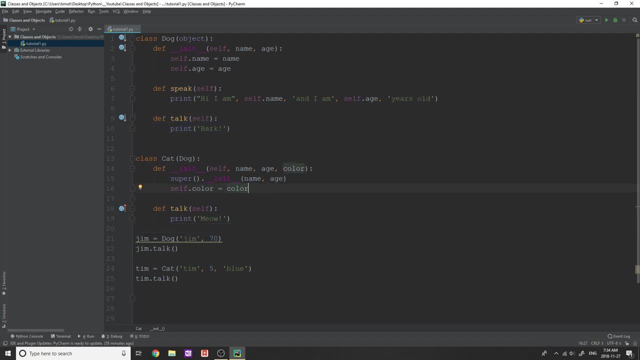 created in doc. And this is the same. if you do something with like these attributes- So if I do like self dot name and I just statically type in a name, like I type tech, okay, Then when we do Tim dot speak now, you would think that it's gonna get: Hello, I am Tim, because that was the 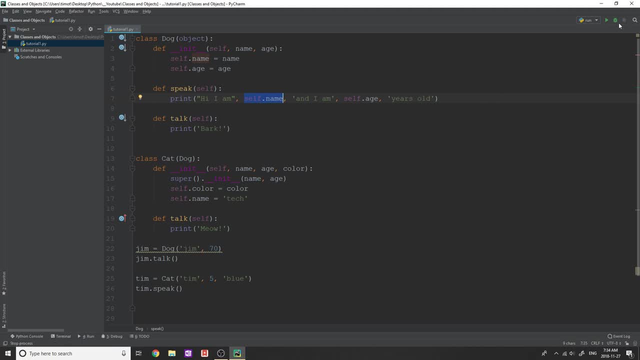 name right And I am five years old, but instead we're going to get tech. So it says: Hi, I am tech and I am five years old. And that is because, although we set name up here to be equal, 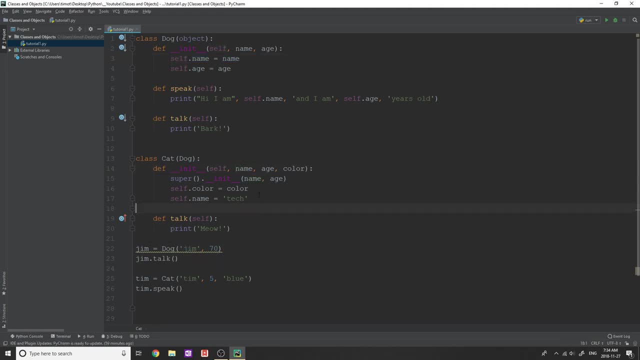 to whatever name we type in the in as a argument. we are changing it to tech and that overrides whatever happens in this dog class. Okay, So I hope that makes sense. Now, what else can we override from those classes? Well, we can inherit like multiple times. we can inherit different. 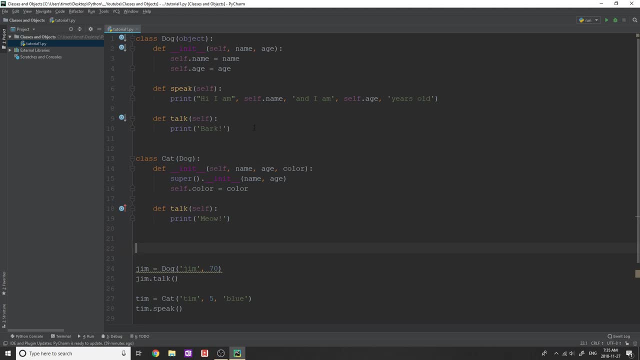 classes from upper class. I'm going to talk about the way you'd want to do an inheritance. Okay, so the way you typically want to inherit is you want to have one really general class, that kind of applies. that's a bit smaller, that applies to like a bunch of 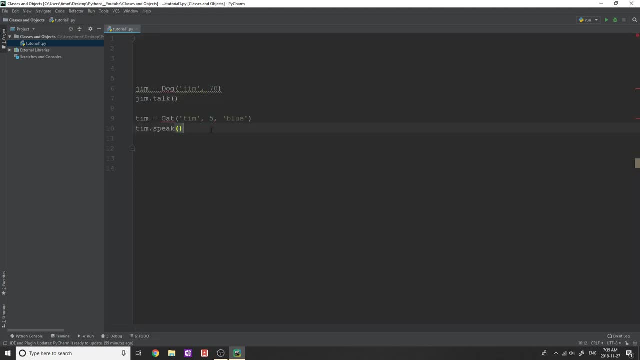 different classes. So I'm going to delete these and I'm just going to type out them and show you an example of what I mean by general class. So if I created a class and I called it vehicle like that, okay, is that how you spell vehicle? I don't care, We're just gonna leave it like that, Okay. 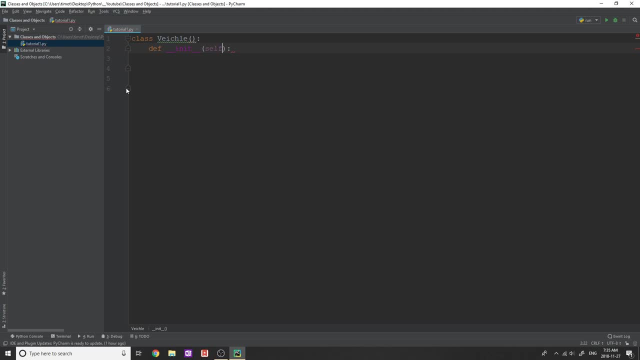 And then I created an initialization in here. Okay, and the initialization is going to take like: price, gas and color. Okay, I know these are random, but just follow: self dot price equals price, self dot gas, gas and self dot color. 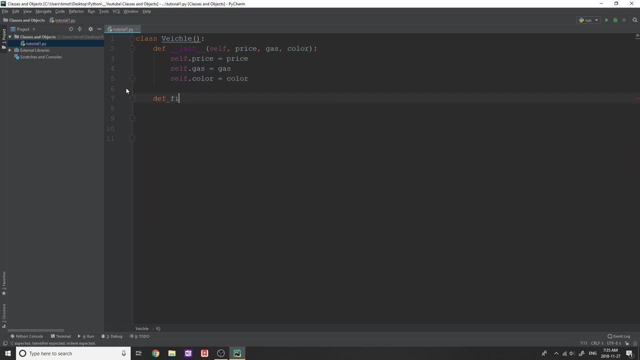 equals color. Okay, now I'm just gonna give it a method I'm going to call define fill up tank like this: Okay, And what's going to say? a self dot gas equals, and we're just gonna say that each gas tank has a maximum of 100.. Okay, let's say: define empty tank, And this is just gonna say self dot gas. 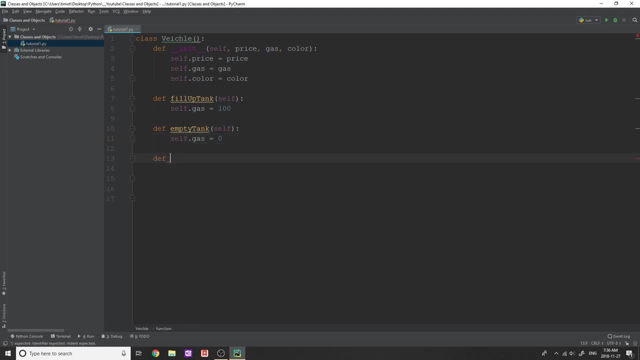 equals zero, And then we're gonna say: define gas left And this is simply going to return self dot gas. Okay, And the reason I have this is because, well, in all vehicles we're probably going to want to have gas. right, All of our vehicles are going to have gas, if they're not electric, obviously. 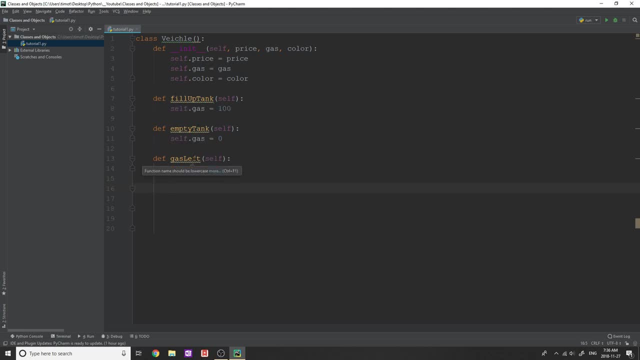 we're not going to deal with that for now. So fill up tank, empty tank and gas left is probably something we want to know for all of our different vehicles. Now, for example, if I create another class, I say class car- okay, And car is going to inherit from vehicle like that, Okay, And all we're going. 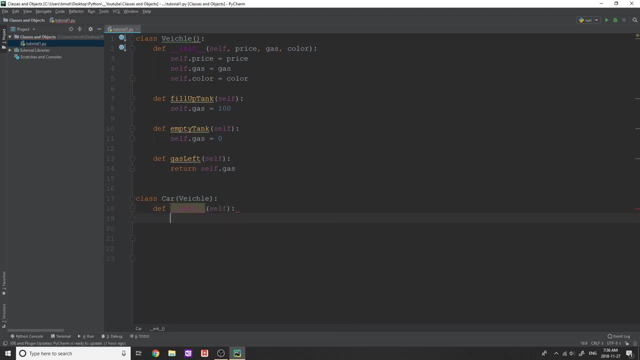 to do for the init is we're just going to call the vehicle in it. So how we do that is super dot, underscore, underscore and underscore, And obviously this needs now a price, gas and a color. So we're going to pass it: price, gas and color, like that. 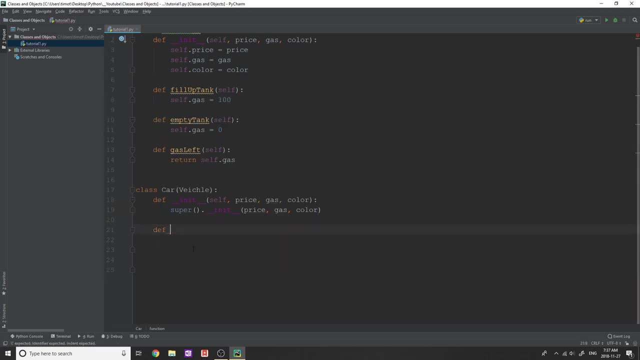 And then that's our initialization, And in car, all we're going to have is we're going to have a method and it's going to call: let's. actually, let's add one more thing here: Speed, Okay, Self dot, speed equals speed, Okay. And then here, as a method, let's just have like beep, Okay And all. 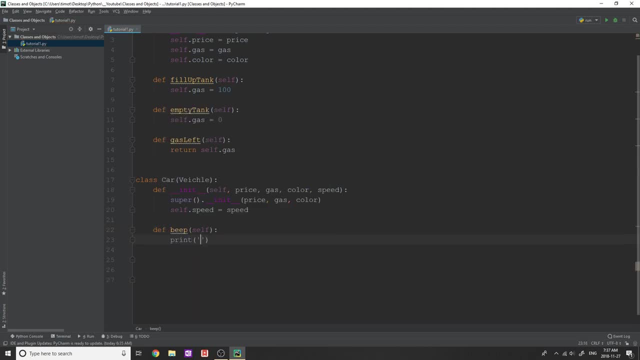 this is going to do is simply print beep, beep Okay. Now, I know these aren't great examples, but just follow along. So we have now is we have a vehicle class, Okay, And it has these things that do with gas And 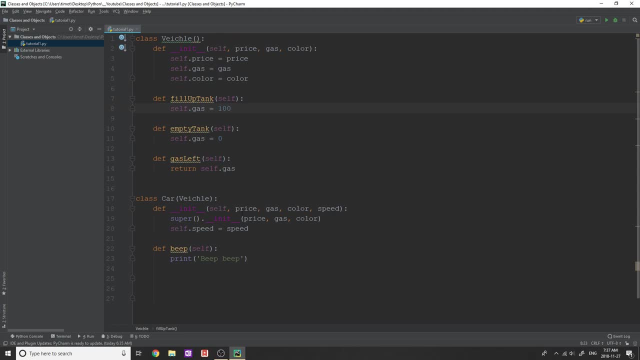 obviously gas is going to work for all of our different types of vehicles. And then we create a car class that inherits from vehicle And in here all it does is it has an extra attribute called speed and it has a method called beep. Now, if I create another class instead of car, I want to